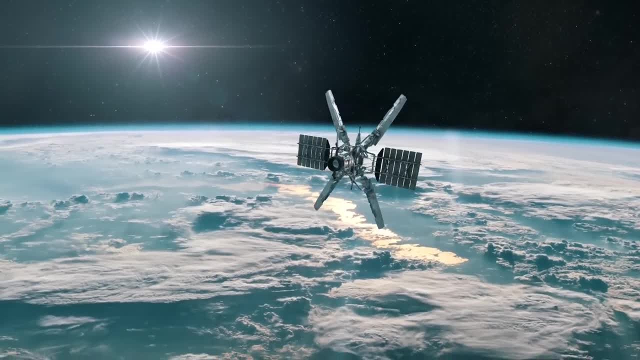 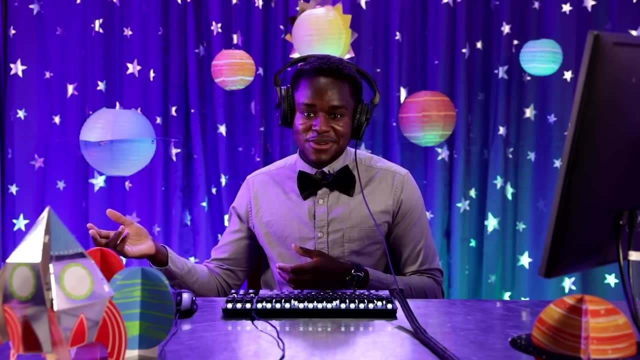 there's on orbit activity, which is where I come in, where we're tracking the satellite or the spacecraft, 24, seven, And then the last stage of the space life cycle is the orbit where we're trying to bring it back down to you know. 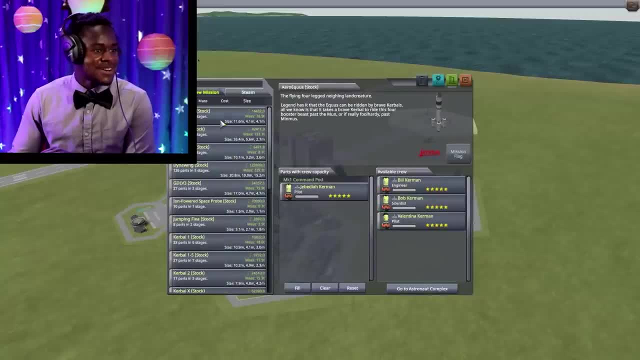 prevent space junk and all that kind of stuff. So I'll start easy for now The GDLV3.. Geez, Okay, Always so many acronyms and like the space world and it's absolutely ridiculous. So we got the solid fuel boosters, protective shell- Okay, And that's going to help. 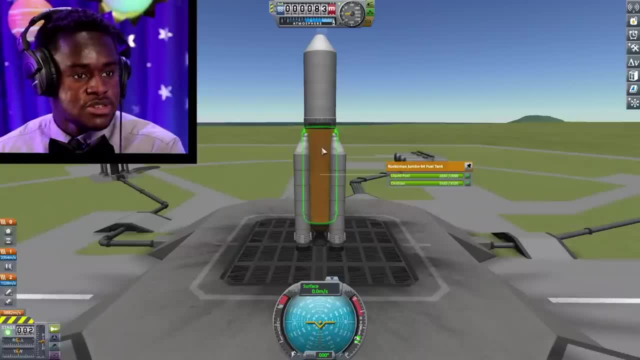 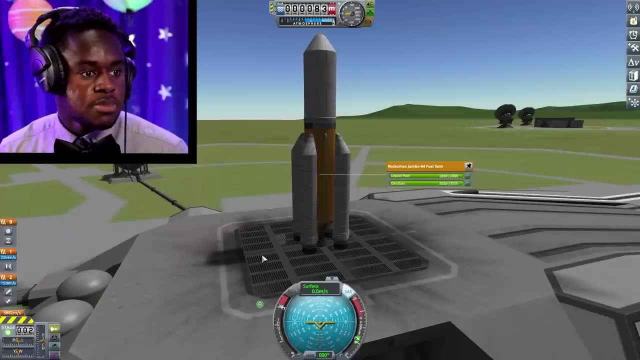 us. This protective shell is going to help us be prevented from heat damage. I'm going to try to launch. It might totally blow up on my face- and launch. Let's see what this bad boy does. All right, So it looks like we've left the ground. I haven't crashed yet, So I'm 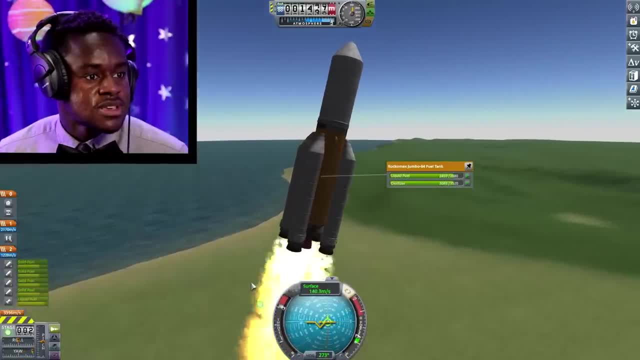 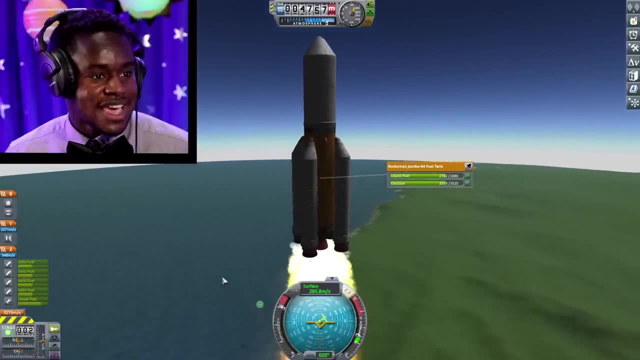 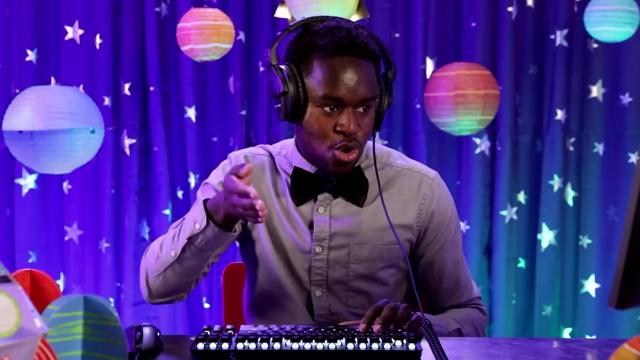 pretty proud of myself. So right now I'm adjusting the yaw a little bit. Yaw is so there's three sort of kind of like the X, Y, Z, access. There's three sort of directions, I guess, or frame of references. So there's hitch, roll And then yaw is like your left and your right. 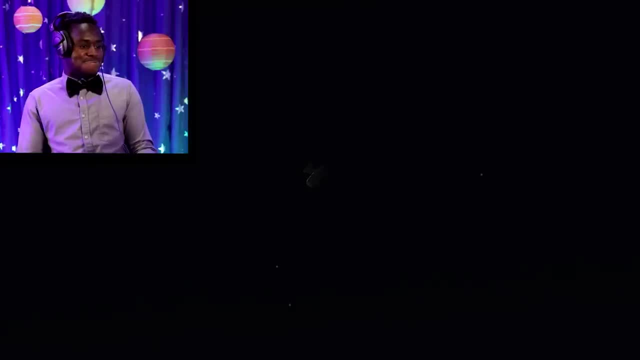 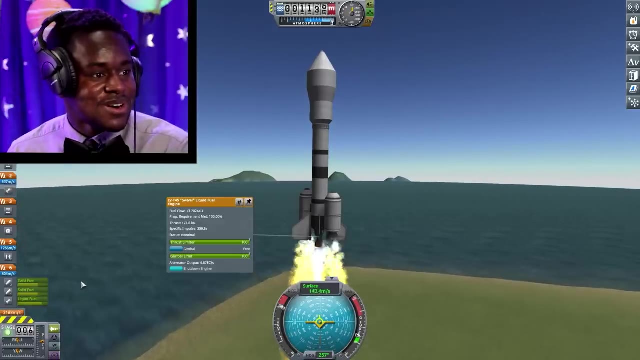 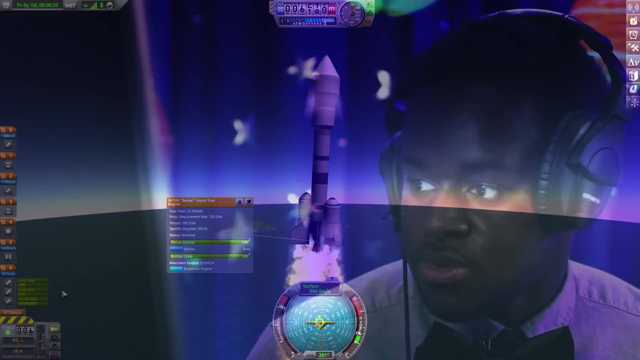 Yikes, Okay, Hey, at least no one died. Okay, So we are all clear. Looks like the fuel meters are going down, which is good. Everything looks nominal, which essentially means normal. So it looks like we just release the solid boosters because we no longer needed them. They were out. 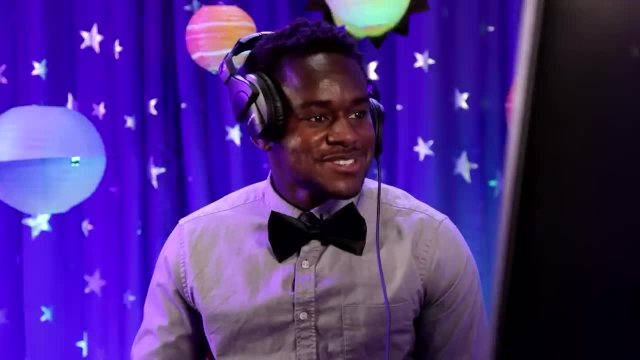 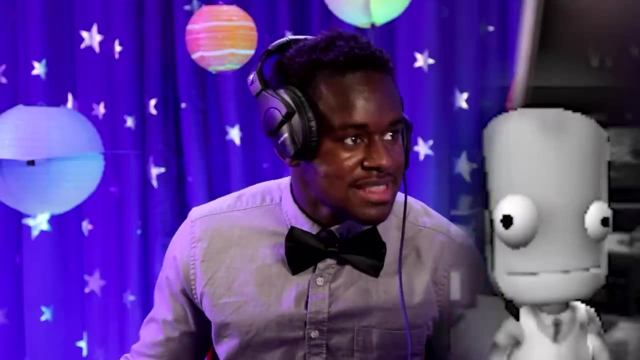 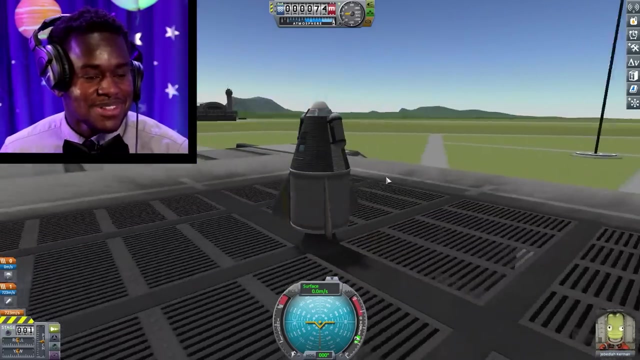 of fuel. Oh, oh, oh Okay. So let's try something a little different. Let's up the stakes And, uh, put these little Minion. things lives at stake. This is exciting, but also kind of nerve wracking, because I really don't want to let Gemadaya down. You all see the way. 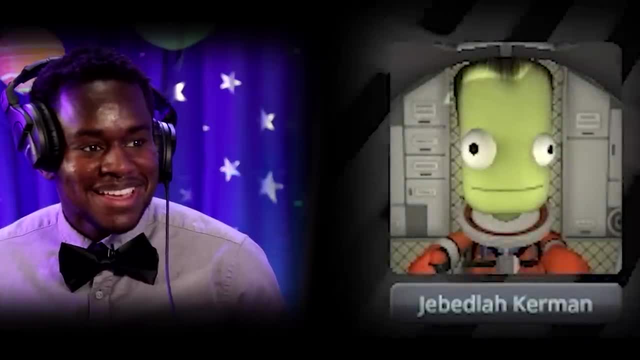 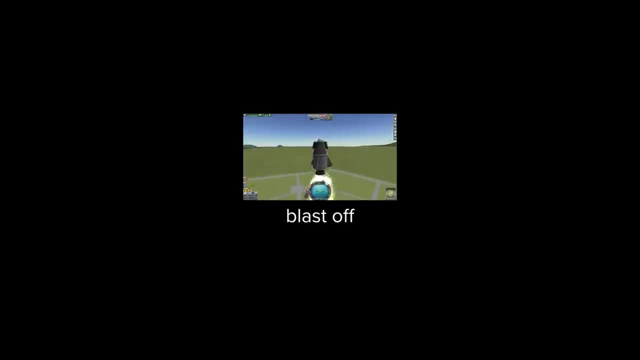 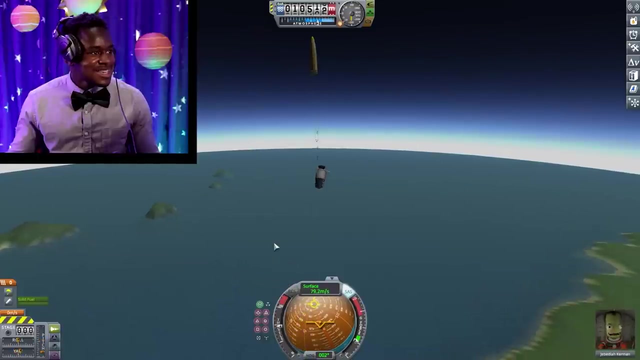 he's looking at me right now. Three, two, one Blast off. Oh yeah, Gemadaya. Gemadaya looks like he's doing good, So I'm really happy. He looks happy, I'm happy. I think it'll be a nice landing, yeah. 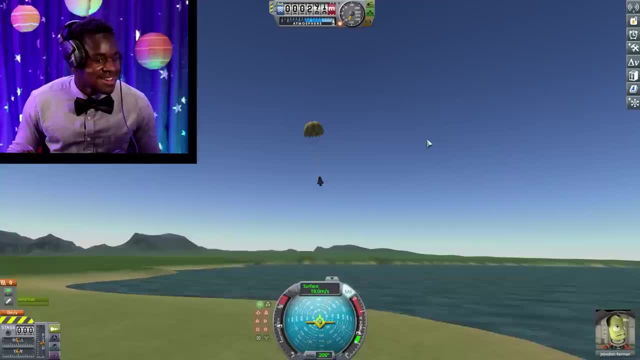 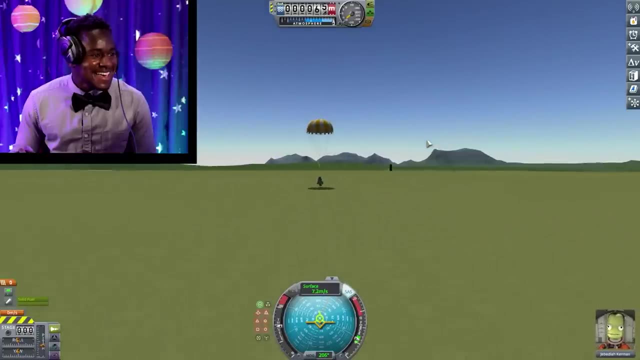 I'm excited to see this pan through. Jebediah, I got you, Don't worry about it. buddy About to land here. Oh, this is perfect. Yes, I am super proud of myself. Hey, Jebediah's clapping for me too. 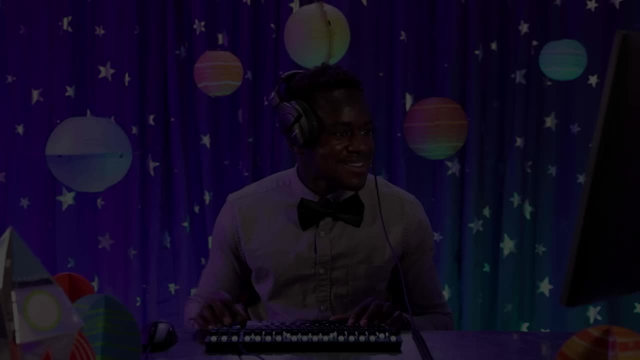 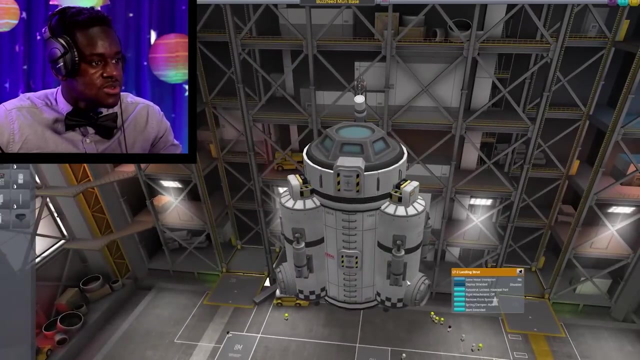 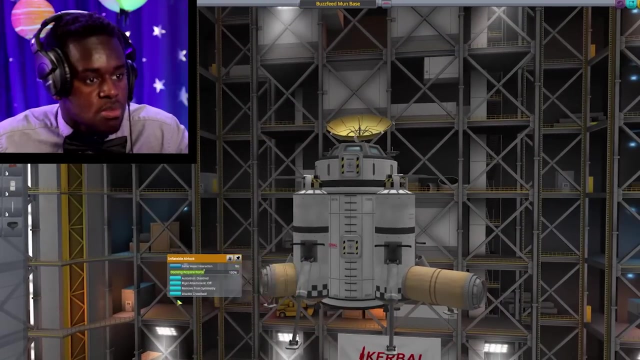 Thank you. All right, Hey, that was successful. That was great. All right. so we've got our module here. Showing you guys the different parts: These are the air locks. so these are really important so that the actual module is not exposed to the harsh environment. 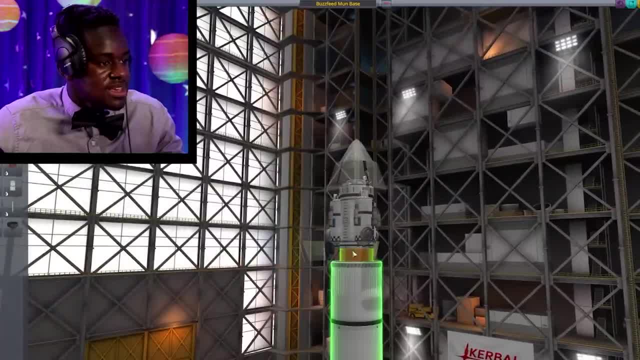 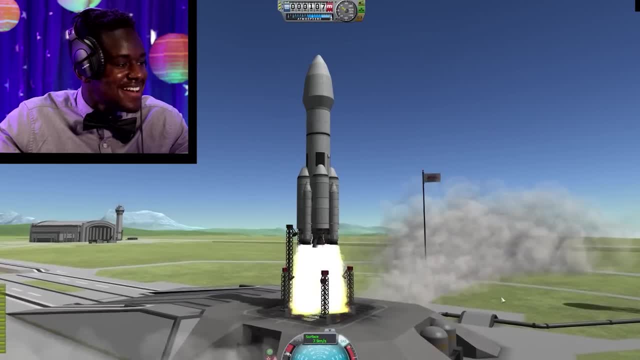 All right, now let's connect the rest of the body and I think we're ready to launch. Then let's get ready to launch. All right, We are burning through that solid fuel body Pretty quickly here now. Bye, everybody. 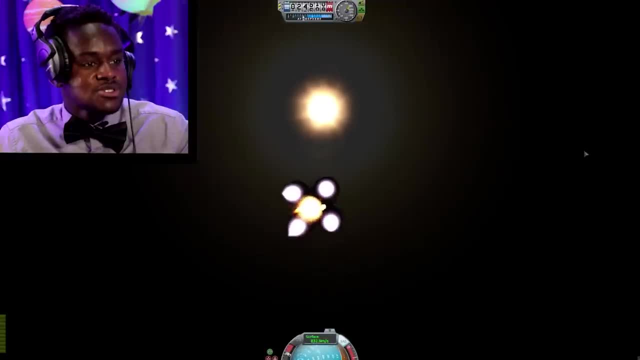 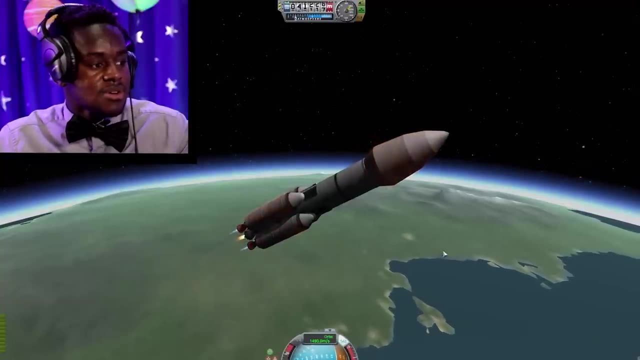 See, y'all never All right. Very cool. Look at those thrusters, Look at the sun. Oh my gosh, This is really cool. So now we are leaving Earth's atmosphere. Let's see, also checking the different orbits here to make sure that we're going to the correct place. 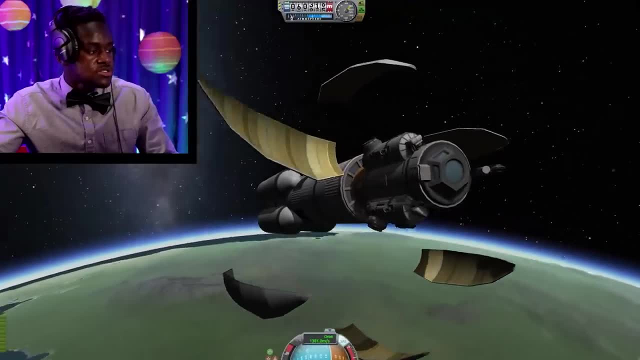 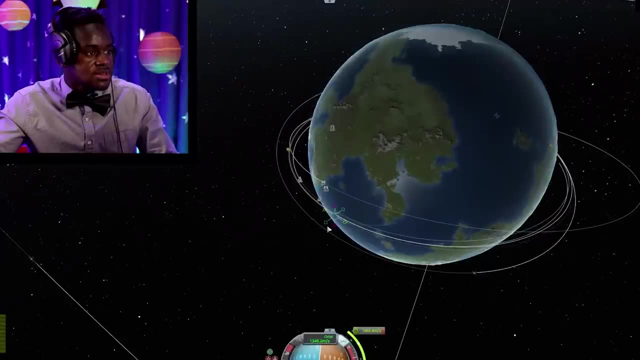 Now that we're actually in the atmosphere, we can dissolve this protective shell. Now, in order to actually go to the moon, we're going to have to Get the maneuvering correct. Here we go, Here we go, Here we go. 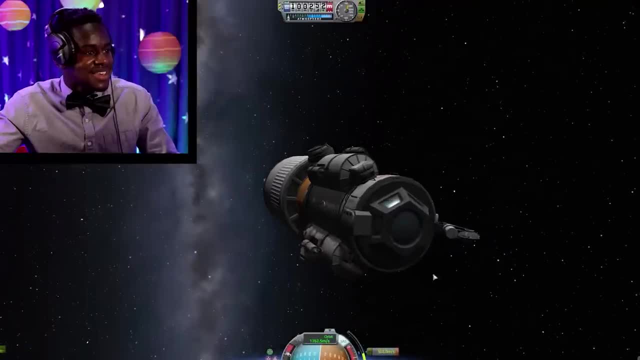 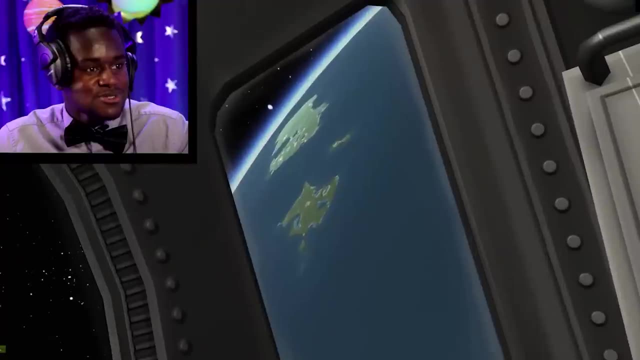 Oh look how pretty that is. Ah yeah, I've always wanted to go to space. honestly, There's Dudo giving us a first look of what the inside of the module looks like and what Earth looks like from space. And, of course, we have snacks. 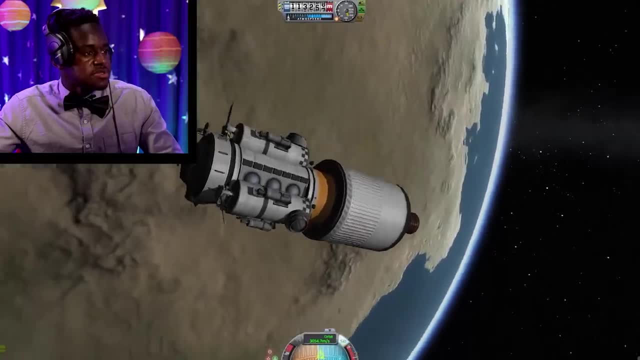 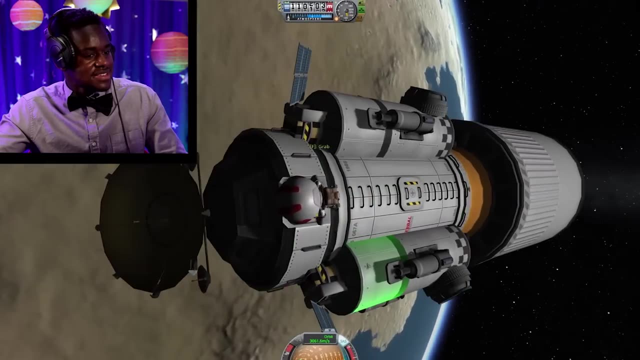 There's a lot going on in this game. I love it. It's just beautiful, honestly Peaceful and quiet. Let's let Dudo over here get some EVA time- extravehicular activity which is essentially spacewalking. 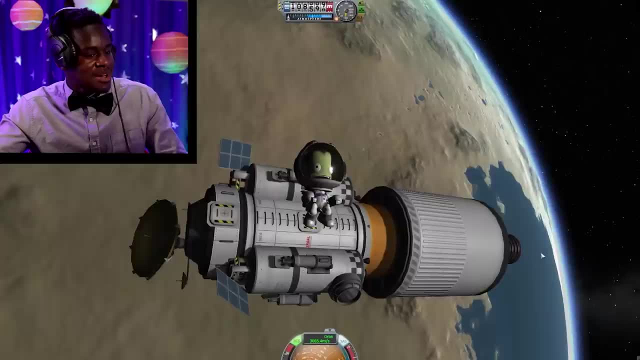 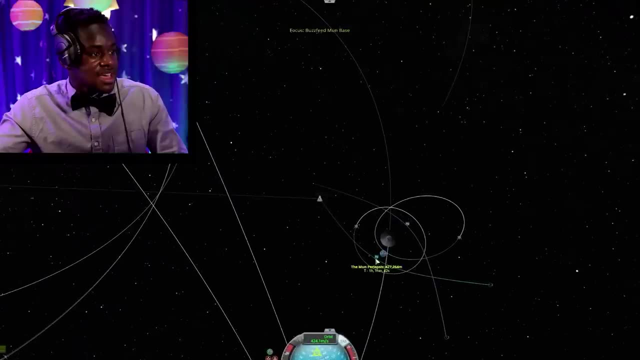 But he's not really walking right now. He's just kind of chilling. I would not recommend any human do this, because this is pretty unsafe. But we are in the moon's orbit and now we just need to land safely. Now let's turn on those thrusters. 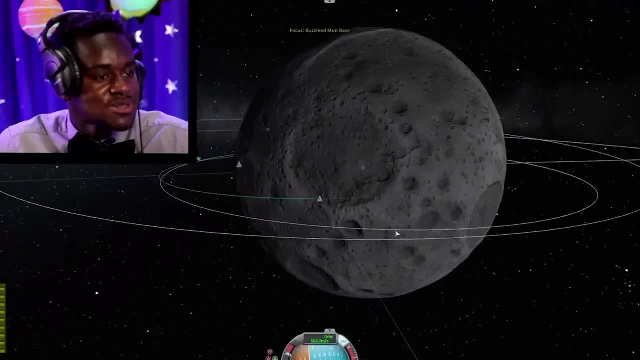 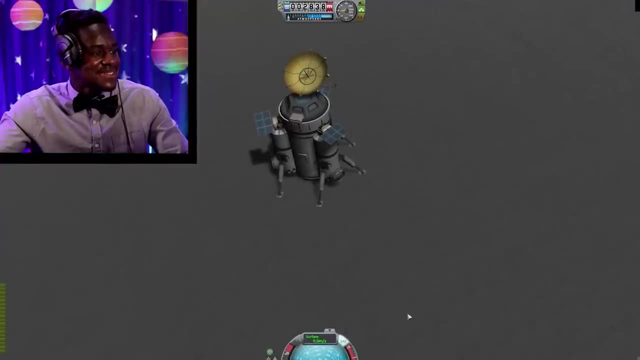 We're going to try to make as gentle of a descent as possible. There we go, There we go, There we go. Yes, Let's come and habitate on the moon. We are doing it, Dudo. Now let's give Dudo a chance to walk around. 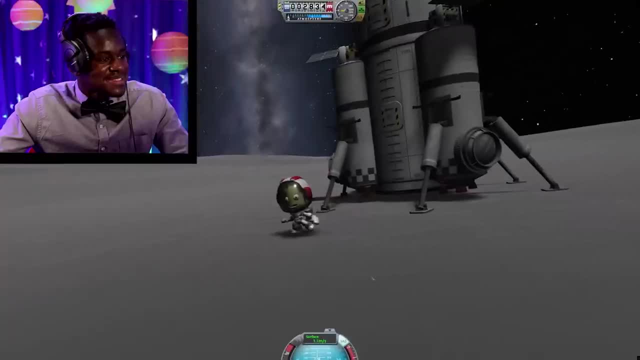 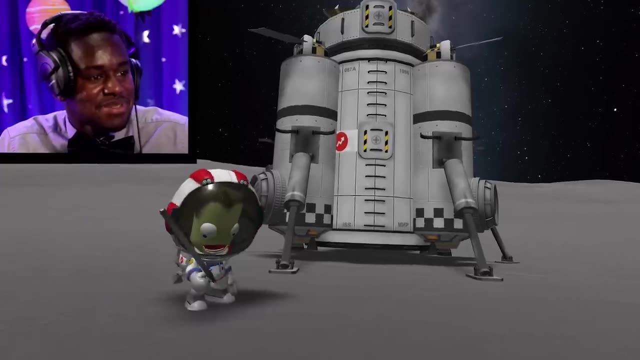 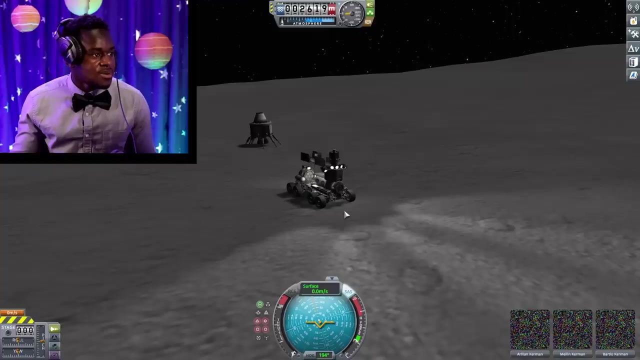 Look how happy he is. Y'all. this is what makes this all worth it. After all the struggle, just seeing him like this, it's all worth it. Time to plant the flag: USA, USA, USA. All right, We are on the moon. 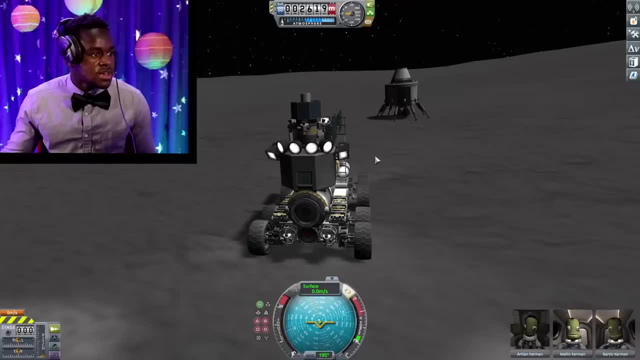 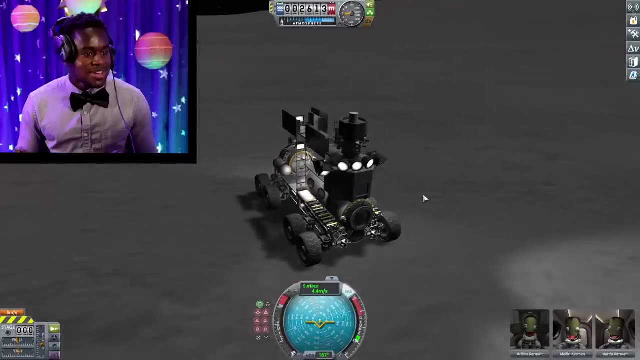 And we got a whole new crew too. Hey, Here let's try to explore what the moon has to offer. As long as the crew's having a good time, I'm having a good time And they look happy- A little too happy actually. 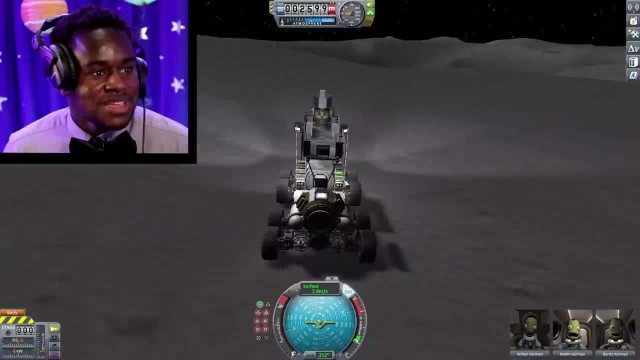 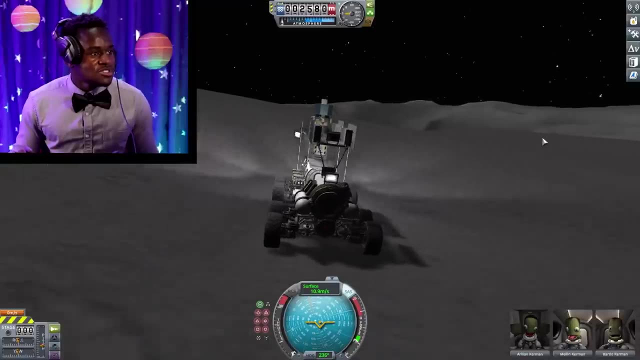 I don't know why their mouths are open like that. I don't really have a goal in mind at this point, I'm kind of just exploring. So yeah, it looks pretty much what I'd expect the moon to look like On the actual moon surface. 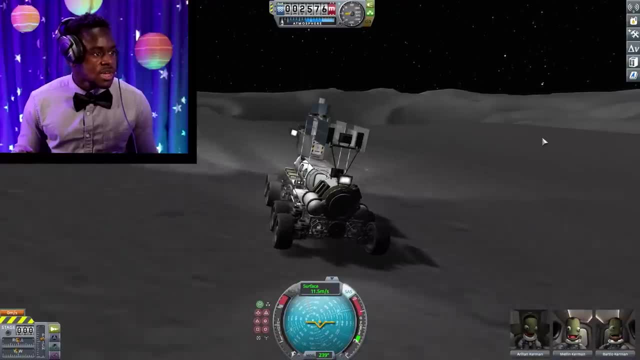 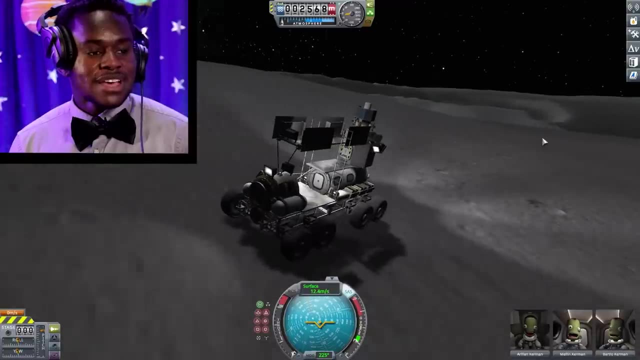 On the actual moon surface. it'd be a lot harder to actually like drive through, Like you'd be going over a lot of huge rocks and stuff like that. The moon actually only has a sixth of the gravity that Earth does. Oh no. I really like the game. It was kind of difficult to navigate. I think it is super pretty to look at. Kind of makes me think of Sims, right. But like the space version, I really like the Kerbal characters. They add like a little touch of like silliness to the game, I guess. 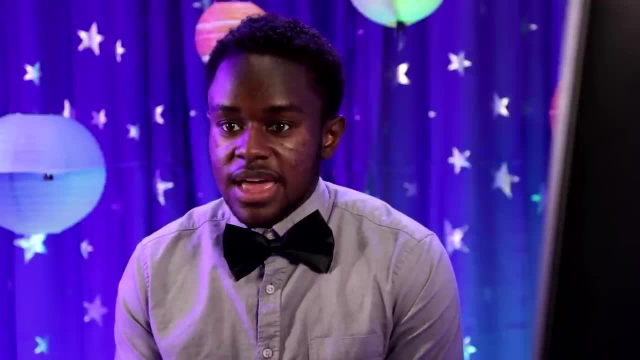 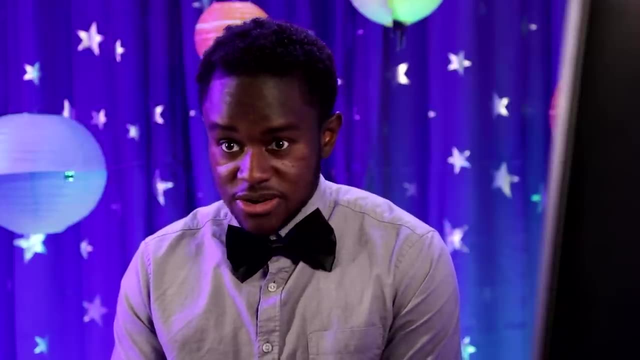 Given that I only get to work with satellites, I think it's really cool to be able to like have a space where I can, you know, see how rockets fly. I think this game would be super helpful for anyone wanting to go into aerospace or really STEM in general. 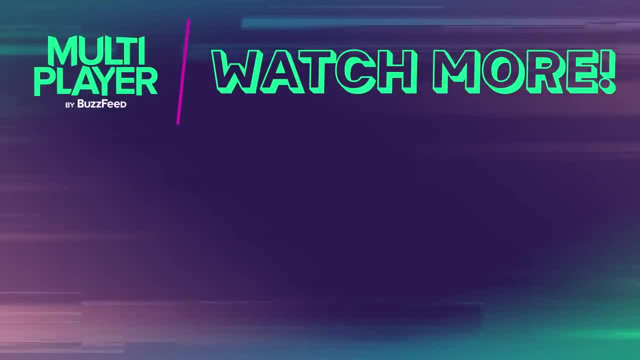 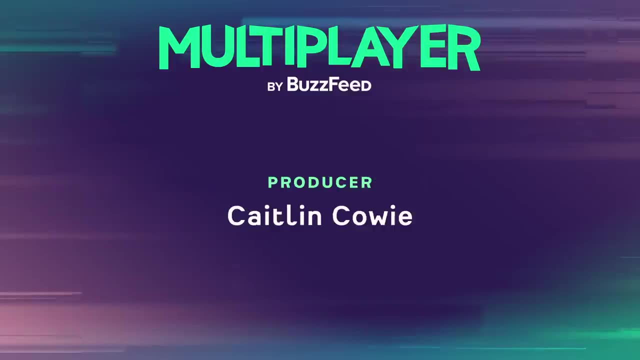 You know, it's just kind of fun and silly And you get to learn about space and rockets in a really, I guess, accessible way. So, yeah, it's really cool. Nice job. Thanks, Mark, Thanks Bri. Thanks everyone, Take care, See you next time. Bye, bye, Bye, bye, Bye-bye, Bye-bye. 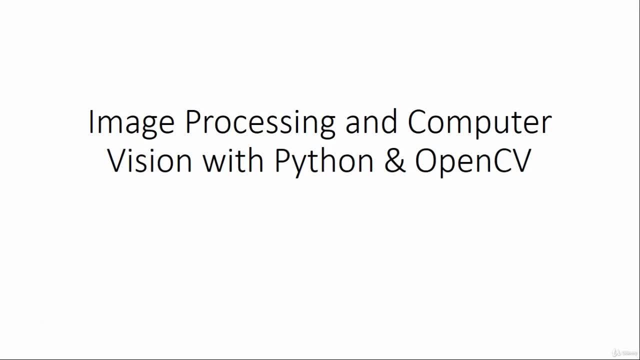 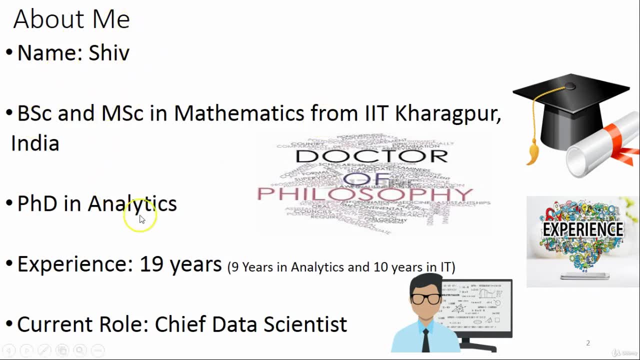 My name is Shiv. I did bachelor's and master's in mathematics, then PhD in analytics and overall around 19 years of experience I have, and last 9 years, in various artificial intelligence area, whether it is machine learning, deep learning, computer vision and so on.